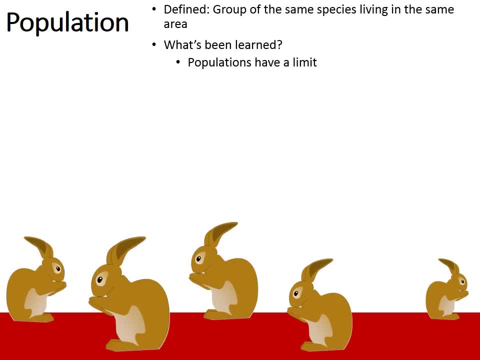 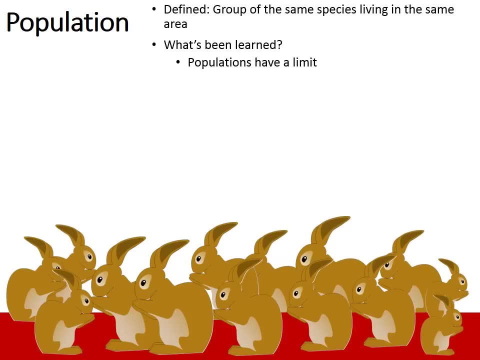 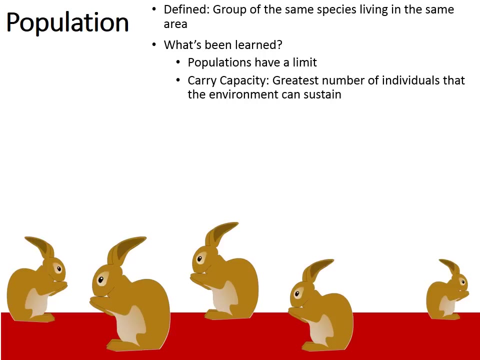 populations have a limit. You know- you may have heard the expression- that rabbits can reproduce like rabbits. They make more, they reproduce in an abundant rate, but there's. what we've seen is that nature limits the amount of reproduction that can occur. What we've seen is that environments typically have or 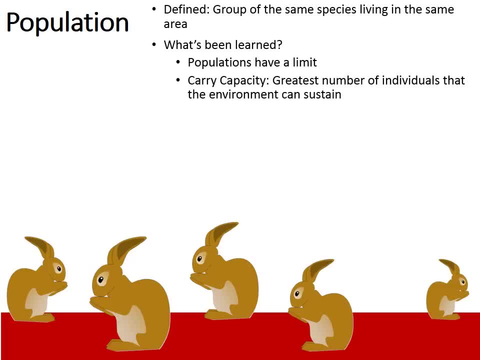 populations typically have a carrying capacity. It's the greatest number of individuals that the environment can sustain. There are limiting factors. There are factors that prevent the overpopulation of rabbits. You know, for instance, there's a lack of resources. Eventually there's just not enough food for all the rabbits to survive. This can. 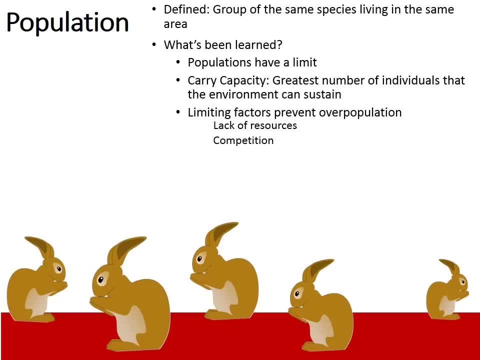 lead to competition: competition for food, for water, for mates, for living spaces, And as populations get larger and larger and larger. more individuals brings more disease, And let's not forget that wherever rabbits live, there's probably predators that are trying to eat the rabbits, and so, for that reason, 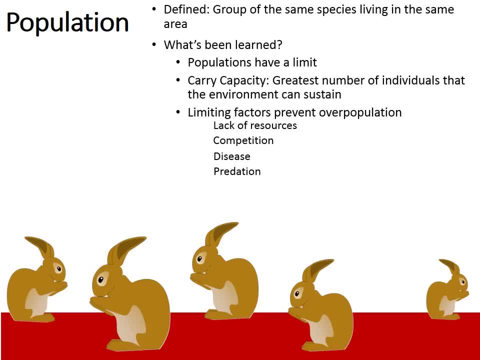 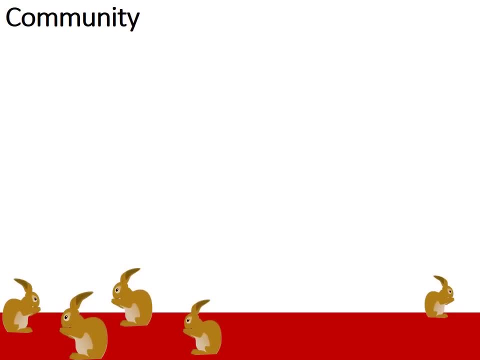 have a limit. They have what we call a carrying capacity. Let's zoom out to the next level of ecological organization. When we zoom out a little bit, we come to a level called the community, and this level is defined as an area where there are many populations living, So not just. 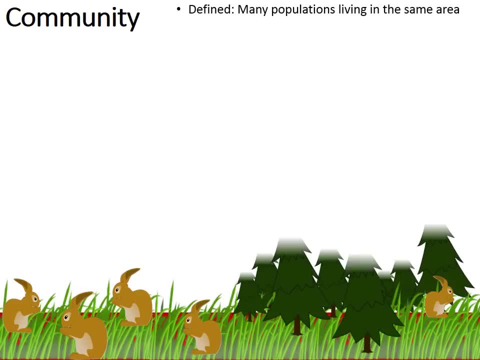 rabbits. also plant life like grasses, plant life such as trees. birds may be nesting in these trees and lurking in the shadows may be some predators symbolized by my wolves. So this is more realistic of a community. And so what have we learned by studying communities? Well, we've learned that each species an 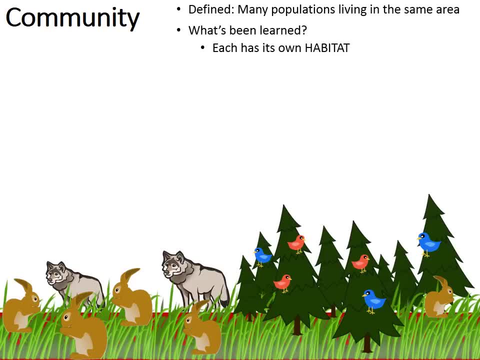 individual has its own habitat. You know, the birds are nesting in the trees, the rabbits are digging through the ground, burrowing and building their homes, And we also learned that organisms have their own niche. A niche is a place where you can find animals that live in the forest. 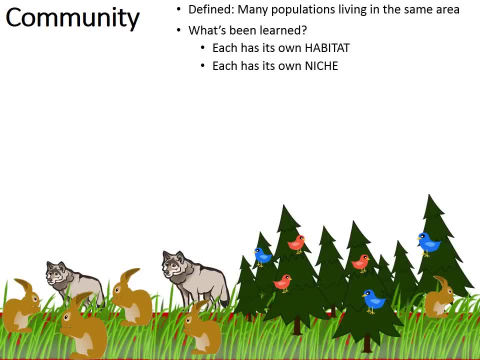 a niche is like a role or a lifestyle that the organism occupies. For instance, the wolves are predators. you know that's their niche. And then you have the rabbits. are herbivores, and other animals that are not pictured here could be omnivores, and other forms of life that are not pictured here could be. 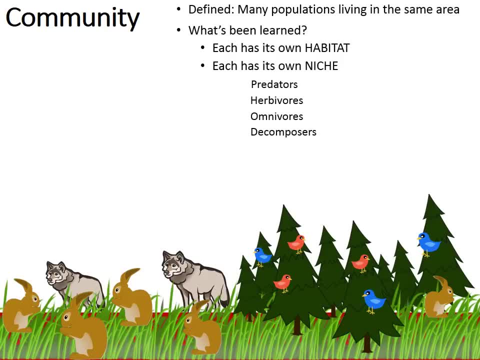 decomposers. You know, one reason why you can have two species of birds living in the same trees is because they have a different niche. The bluebirds, for instance, may build their nest in the autumn months and eat insect A. The reddish- pinkish birds, however, might build their nest in the 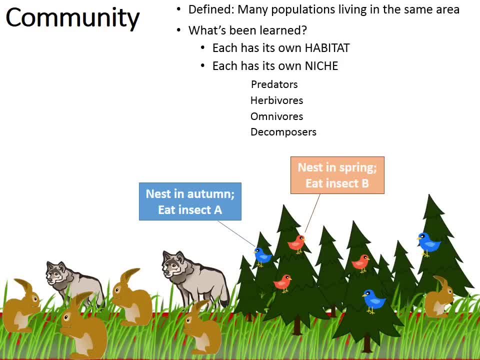 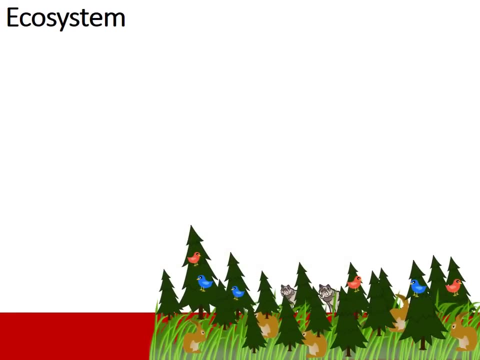 spring and eat insect B Because they're not in direct competition with one another. they're able to coexist. Their niches do not overlap with one another. If their niches were to overlap, you would see competition. If we zoom out, we come to our next level, called the ecosystem. And what's different with the ecosystem? 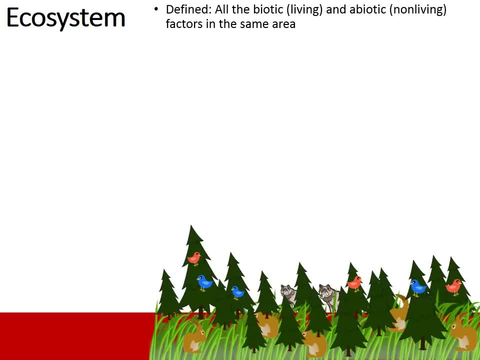 What are we adding? Well, we're adding the living and the nonliving factors in this environment. So right now we have a community, because all the organisms pictured are living, but in an ecosystem, let's say, we add some nonliving rocks. we 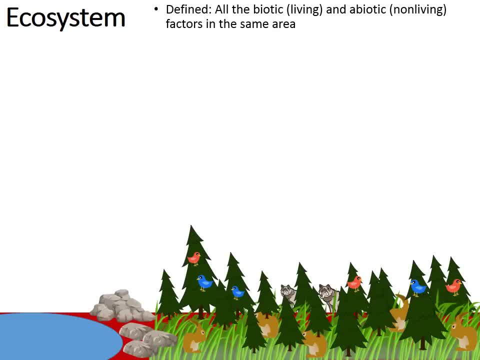 add some nonliving water. now we have an ecosystem, And so what have we learned by studying ecosystems? What we've learned is that the biotic life is affected by the abiotic, which. that simply means that life is affected by nonliving factors. You know, for instance, drought, if there's a time period of extreme. 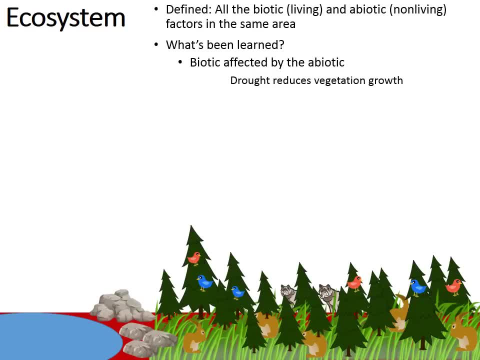 drought. well, this could reduce the ability for plants to grow. Another example would be, for instance, the rocks release phosphorus, which is part of the phosphorus cycle, And so rocks, which are nonliving, release phosphorus into the soil and once phosphorus 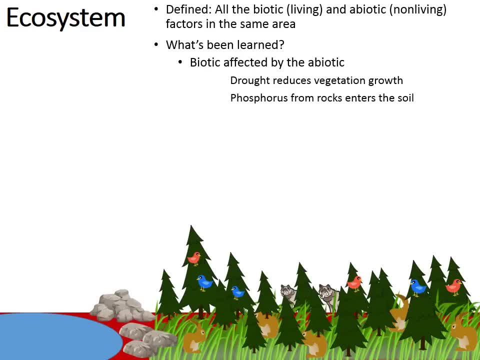 is in the soil, plants can grow and you have it part of a healthy ecosystem. Well, we've also learned that it goes the other way too, is that the nonliving parts of the environment are affected by the living, so the abiotic is affected by. 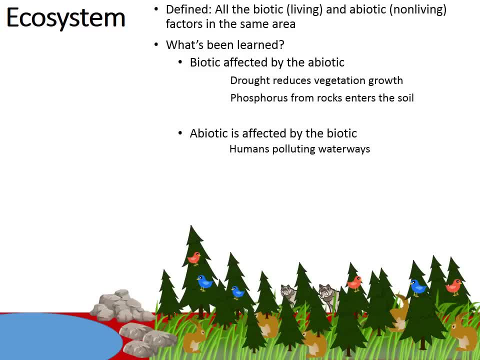 the biotic. Great examples of this would be: you know humans and our polluting of waterways. You know humans, we're a living organism and we pollute nonliving waterways. Another example would be decomposition- a positive example, right? 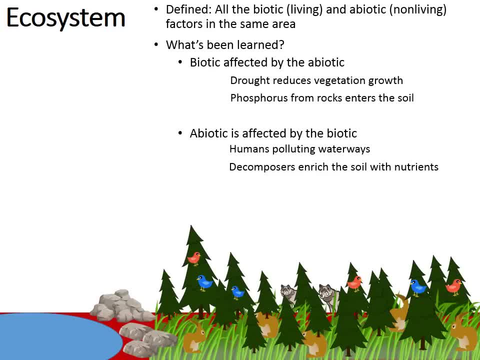 here would be decomposers- living decomposers, bacteria and fungus Living decomposers. they enrich the soil with nutrients. soil is not living, And so these are great examples of how the abiotic factors are affected by the biotic. 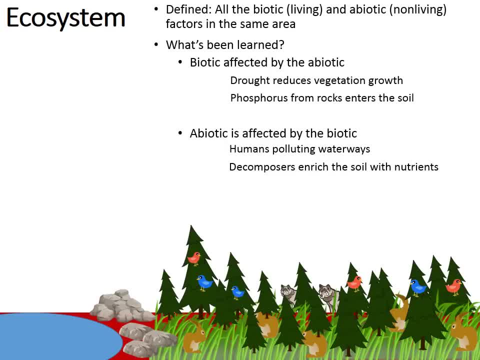 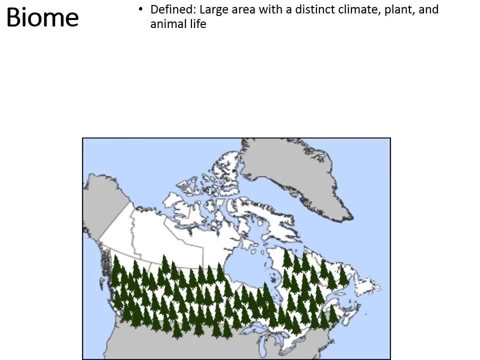 factors. Let's zoom out to the next level of ecology. When we zoom out to the next level of ecology, we come to a biome. A biome is a large area of land with a distinct climate, plant life and animal life. So what have we learned by? 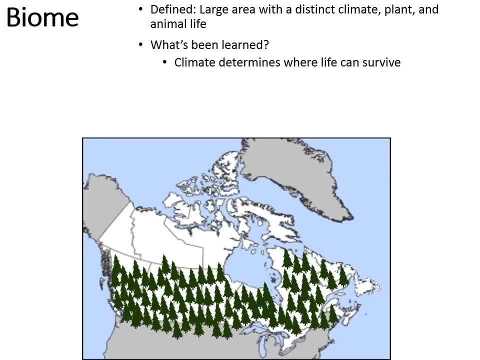 studying biomes, Well, we've learned that the climate of an area determines where life can survive. You know, the biome that you see here- that includes northern United States and Canada- is the biome called the taiga. You know the taiga is. 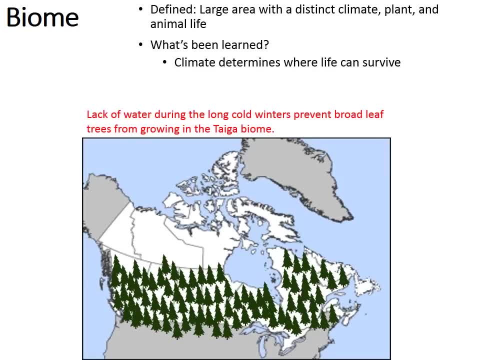 characterized by a lack of water during the long, cold winter months. You know this prevents broadleaf trees and plants from growing in the taiga. You also see very few, if any, cold-blooded animals. You don't really see a lot of snakes and 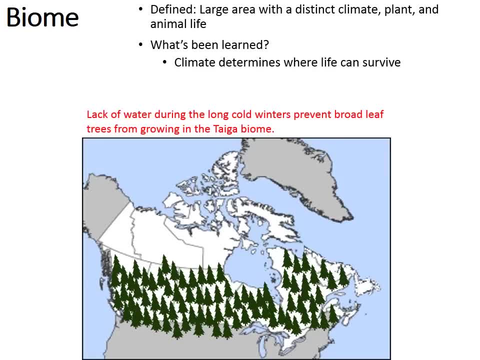 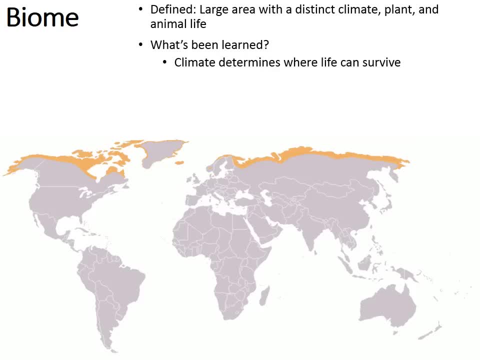 you don't really see a lot of salamanders. Cold-blooded organisms have a really hard time living in these environments. Another biome picture right here is even further north. this would be the tundra, And again, the tundra is characterized by even colder and drier conditions, and this prevents much of any. 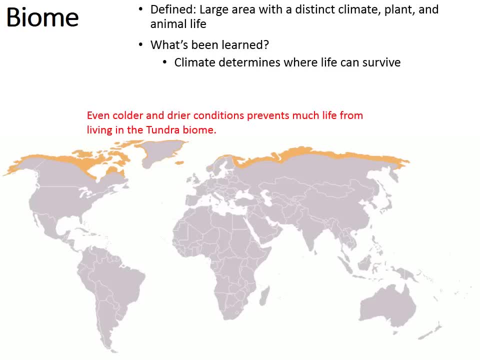 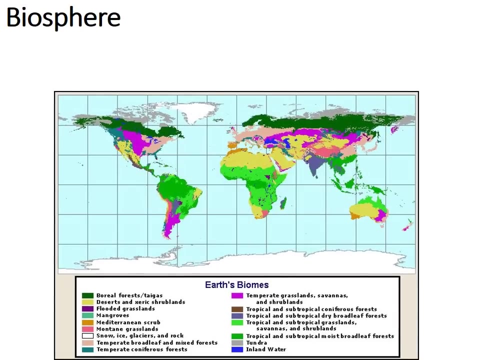 kind of life from living in the tundra. Yeah, you'll see you scatter plants and scattered animals, but for the most part the tundra is a very life is very rare. in the tundra, When we zoom out, we come to the final level of ecology called. 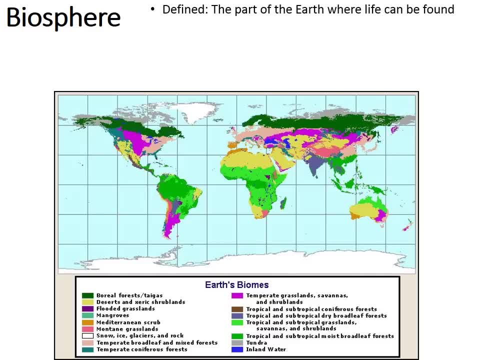 the biosphere. This is the part of the earth where we can find life. You know the picture. here are all the biomes of the earth: the deserts and the tundras and the taigas and the tropical rainforests. You know all the biomes.